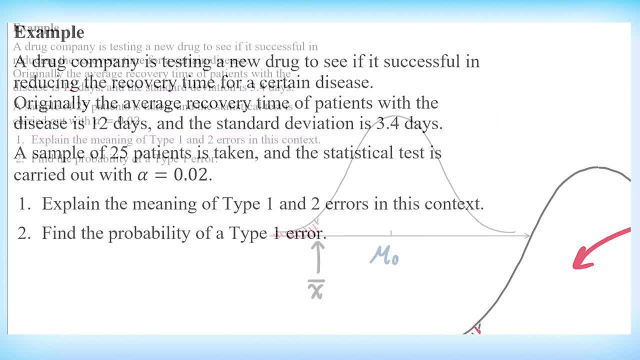 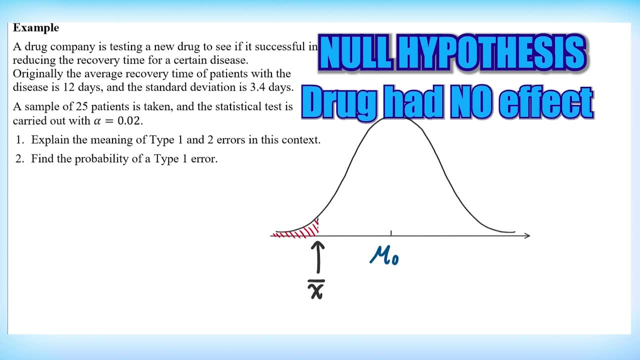 standard deviation is 3.4 days. in this case, the null hypothesis would be null. no difference, the drug had no effect and the mean recovery time of the patients who took the drug is still going to be 12 days. so what would a type 1 error be? well, the null hypothesis needs to be true. so the drug 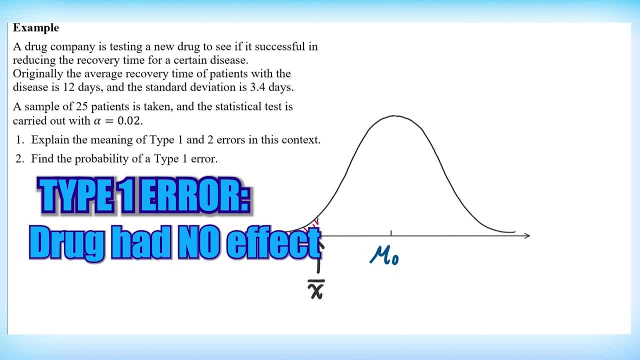 should have no effect, but we need to make an error. so in our test we concluded that the drug did reduce recovery time, even though it did not. that's a type 1 error. the type 2 error is the opposite, in that the drug did recuse, reduce recovery time, but we concluded that it did not. 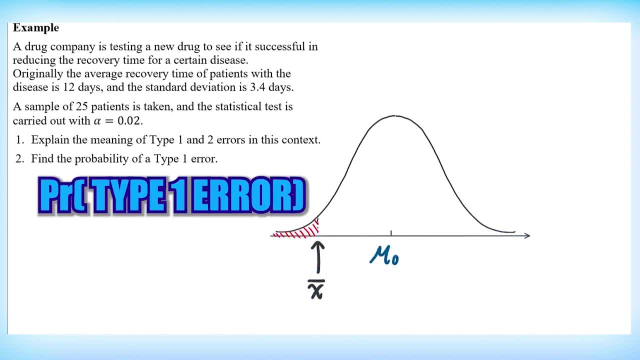 to find the probability a type 1 error occurs. it's actually very simple. it's just exactly equal to alpha, the significance level of the test. in this case, that's two percent. so the probability of making a type 1 error is exactly equal to zero percent. 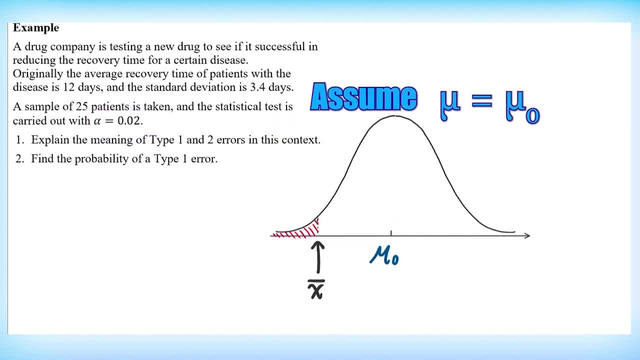 0.02. and that makes sense because if we assume that the null hypothesis is true, the mean is 12. well, the sample means fall on a bell curve around, centered around 12, and if we randomly end up in the bottom two percent, the bottom left tail of the bell curve, we're going to reject the null hypothesis. 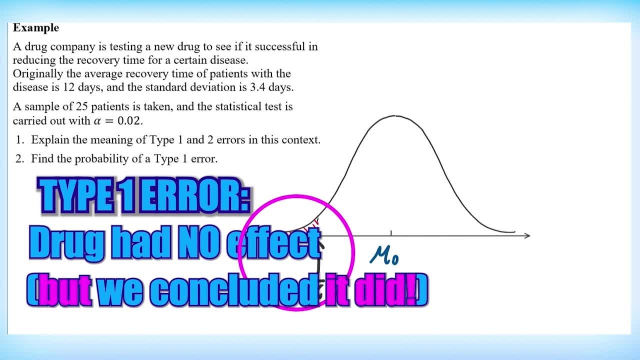 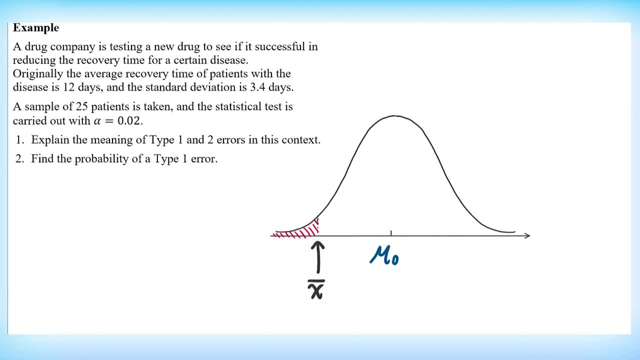 even though it was true we just happened to get a random sample with a particularly low sample mean, just due to random sampling variation. if you wanted to reduce the chance of a type 1 error, well, you could reduce your significance level to say one percent or 0.1. then you would need a. 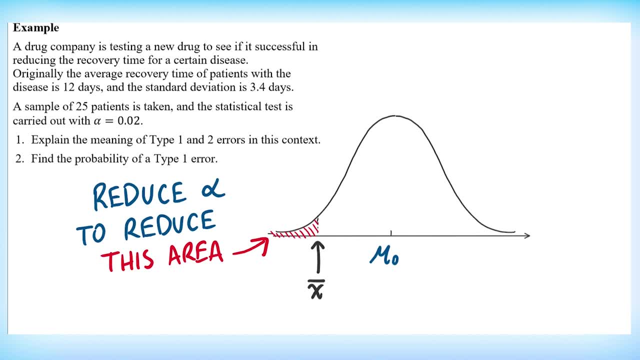 stronger result, a more extreme result of your sample, mean to reject the null hypothesis and conclude that the drug works. so with something like this, with the drug, probably you do want to be quite sure that that drug works and not just have a conclusion based on random chance. so you'd 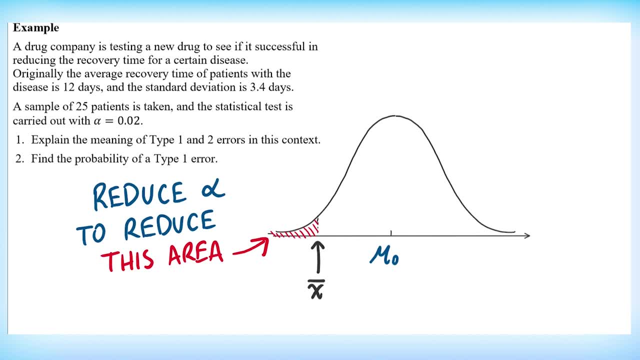 probably be setting that alpha, that significance level, to be quite low now to find the probability of a type 2 error. it's actually a bit more difficult to find the null hypothesis with a type 2 error, because now the null hypothesis is false and we need to find the probability. 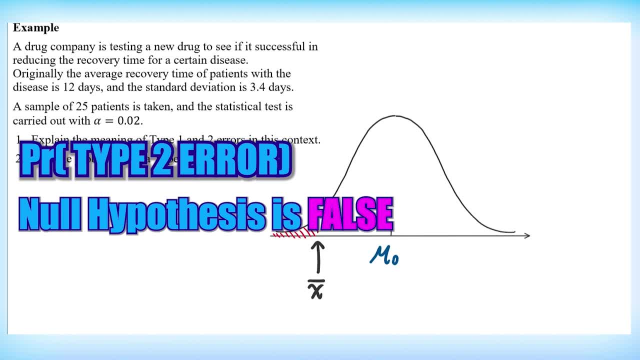 that we did not reject it. but because the null hypothesis is false, we are no longer able to use that mean we were using in the first place and we have to know well what actually is the true mean. so we'll need to be given that in the question. so here's an example: given that the true mean, 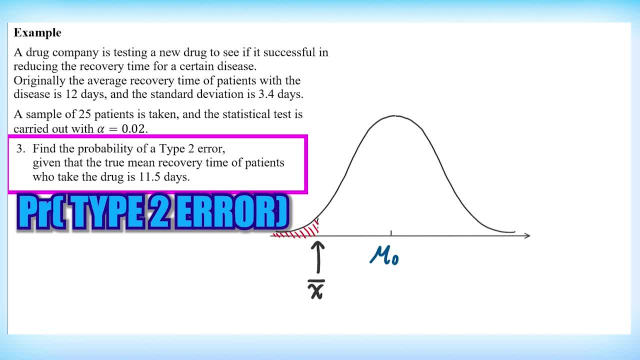 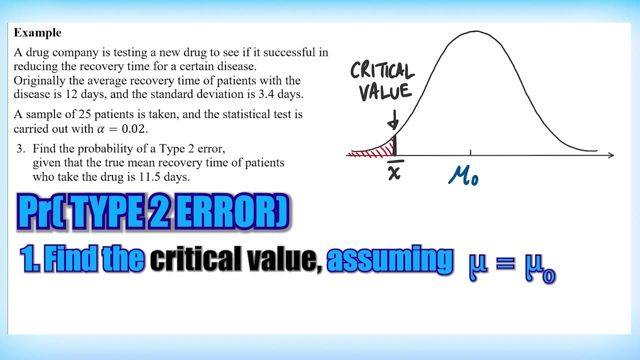 recovery time of patients who take the drug is 11.5 days, not 12, it's 11.5. find the probability a type 2 error occurs. we need to do this in two steps. step one is: given the claimed mean, we need to find the critical value of the sample mean, which would be like the borderline value between. 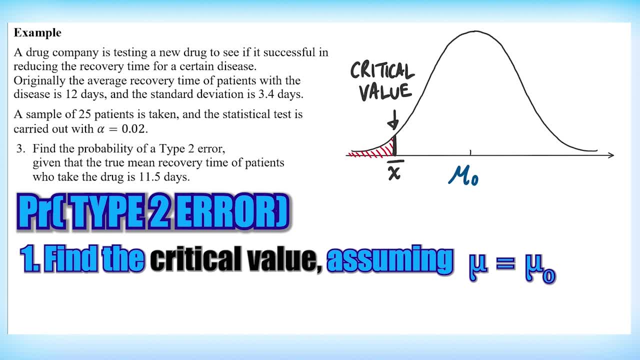 rejecting and not rejecting, and we can find that one using the inverse normal distribution. here's how that looks on the ti inspire, given the claimed mean of 12 and the standard deviation of 3.4 over root n, root 25.. now we know the critical value of the sample. 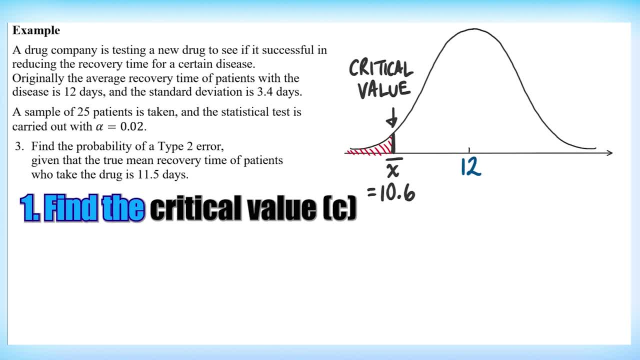 for rejecting or not rejecting is 10.6. so if the sample mean was less than 10.6 we would reject the null hypothesis. if it's greater, we would not reject. now we need to find the probability we do not reject. okay, because in the type 2 error the null hypothesis is false, but we do not reject it. 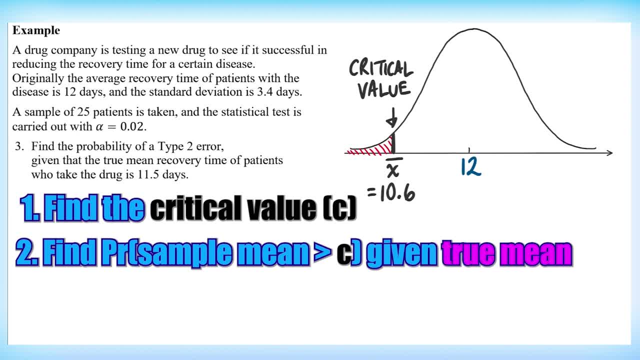 we need to find the probability we do not reject, but not given the original claim mean. given the true mean, okay, the fact, in this case the true mean is 11.5. given that true mean we'll, what is the probability that our sample mean is greater than 10.6? i recommend you draw it up like: 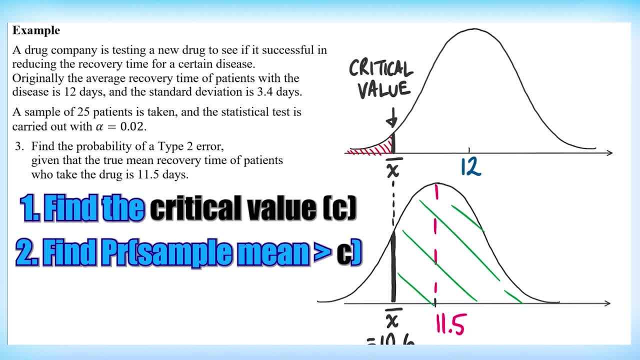 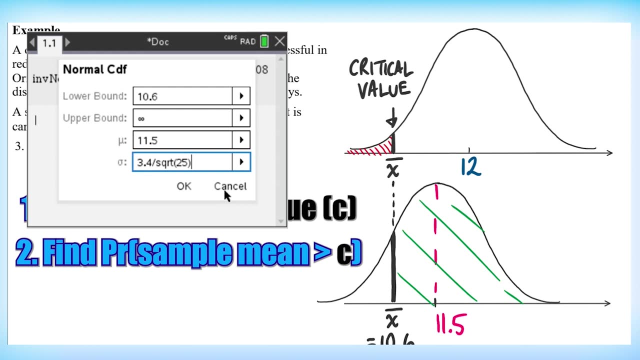 this with two bell curves: the first one with your claimed mean, in this case 12, and once you've found the critical value, the second normal distribution with the value of the true mean. the standard deviations are the same. that hasn't changed, and we just need to find the probability. now that we are 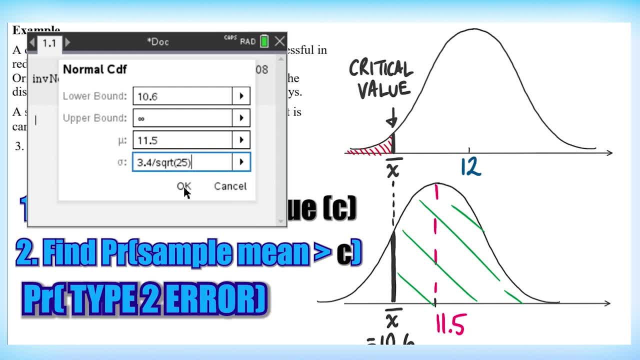 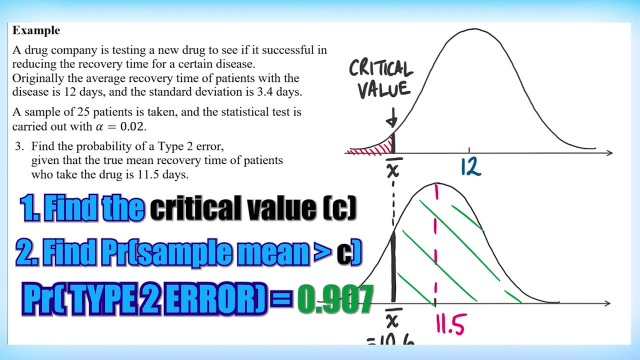 greater than the critical value, in this case greater than 10.6. we're doing a one-tailed test here, with the alternative hypothesis was that the mean is less than 12.. that's why rejecting was to the left and not rejecting to the right. if our alternative hypothesis was the other way, then we'll be in the right tail, and if